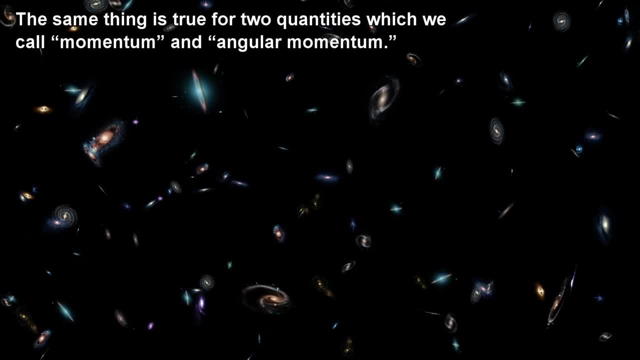 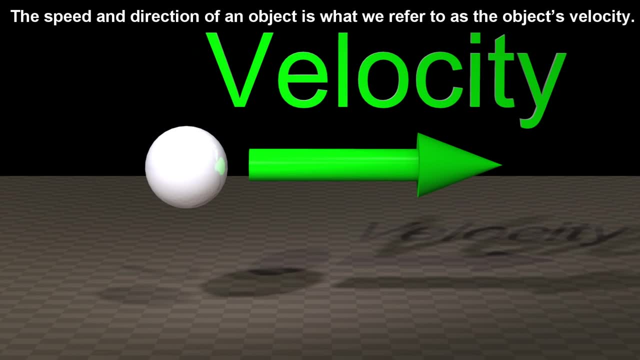 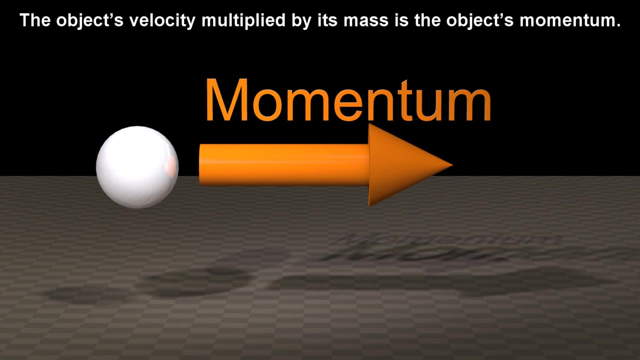 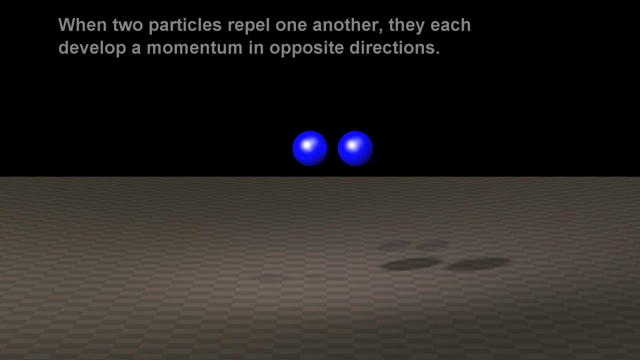 momentum and angular momentum. The speed and direction of an object is what we refer to as the object's velocity. The object's velocity multiplied by its mass is the object's momentum. When two particles repel one another, they each develop a momentum in opposite. 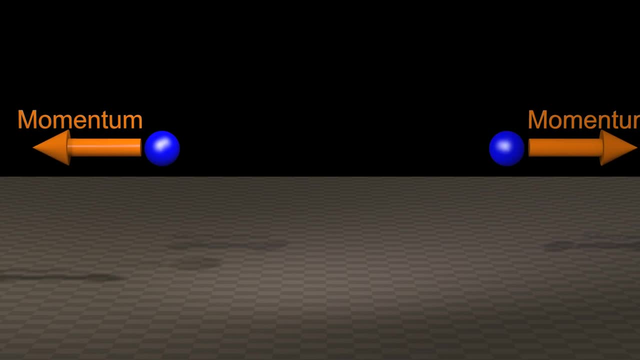 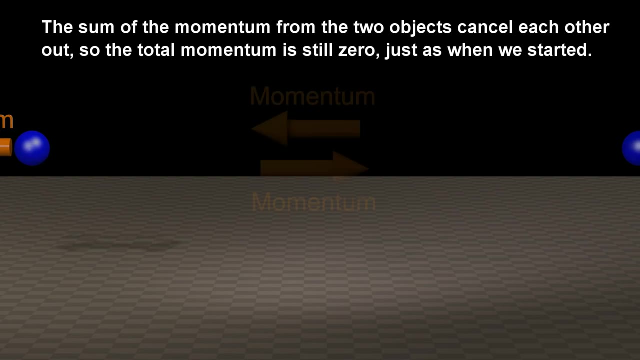 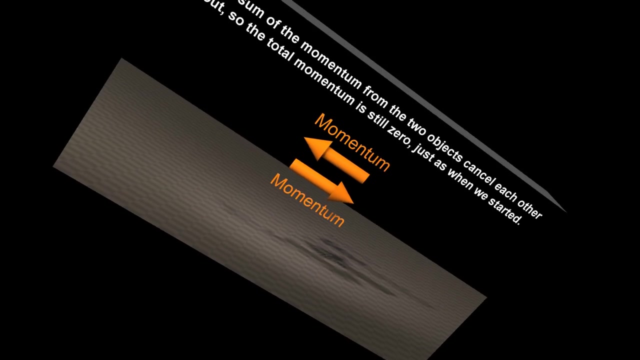 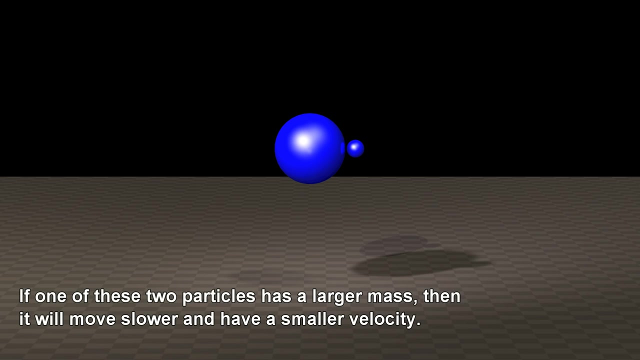 directions. The sum of the momentum from the two objects cancel each other out, so the total momentum is still zero, just as when we started. If one of these two particles has a larger mass, then it will move slower and have a smaller velocity. 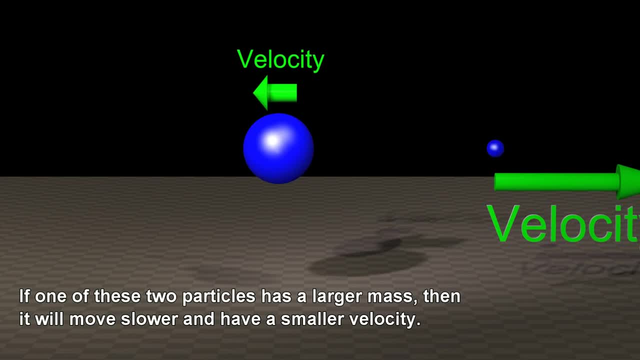 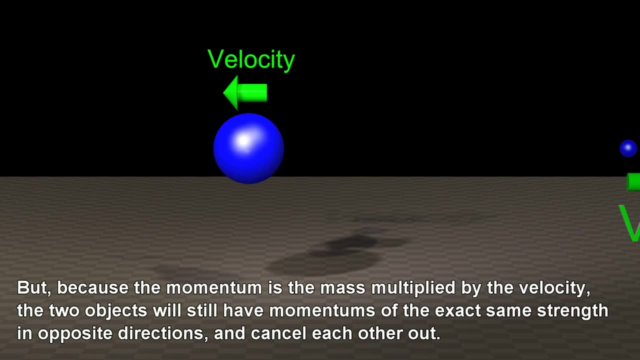 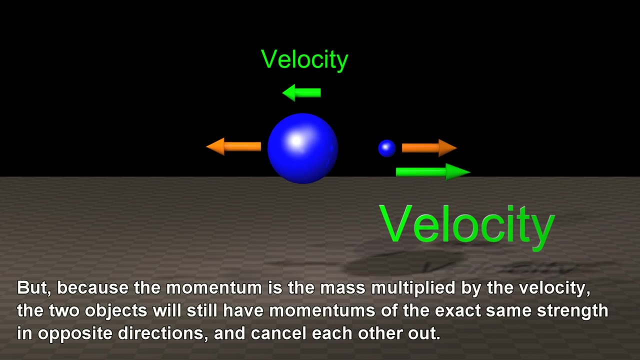 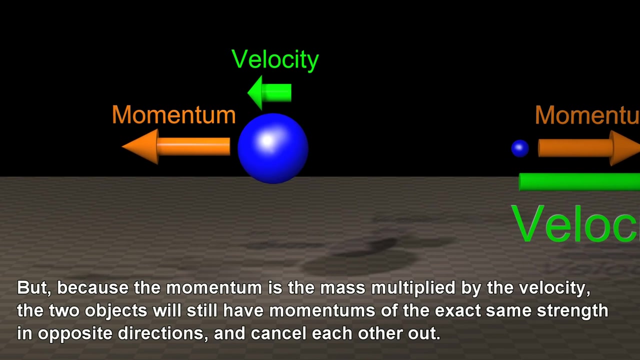 But as the momentum is the mass multiplied by the velocity, the two objects will still have momentum of the exact same strength in opposite directions and cancel out each other. The powertrain of a yak will always have momentum of the exact same strength in opposite directions. 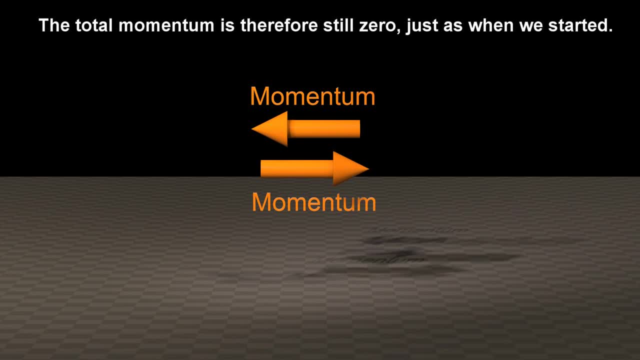 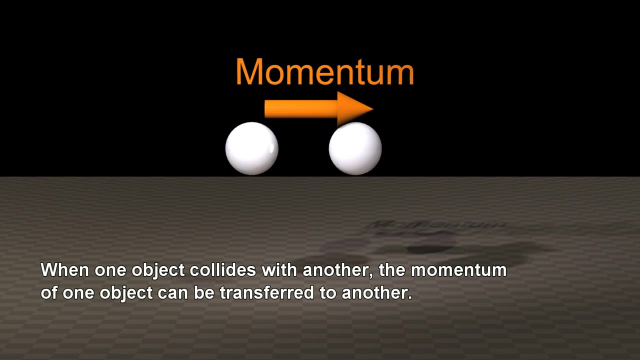 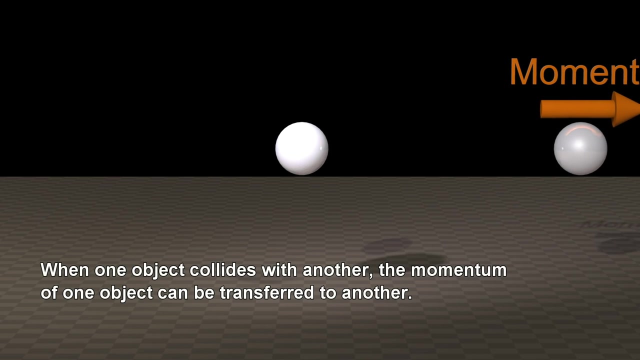 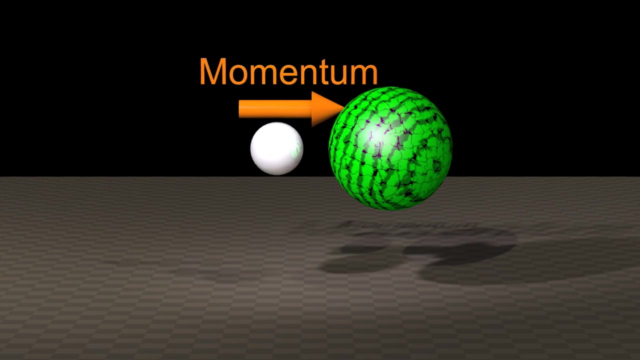 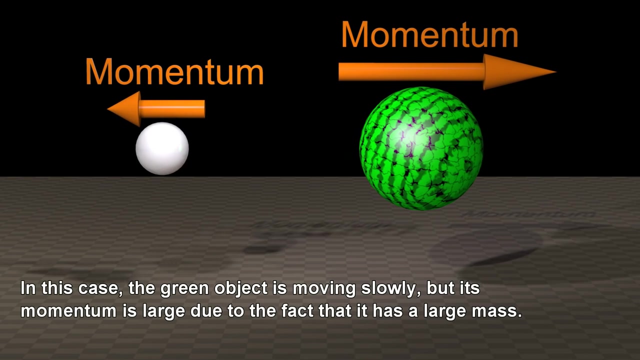 saç ov ç ca. The total momentum is therefore still zero, just as when we started. When one object collides with another, the momentum of one object can be transferred to another. In this case, the green object is moving slowly, but its momentum is large due to the fact that it has a large mass. 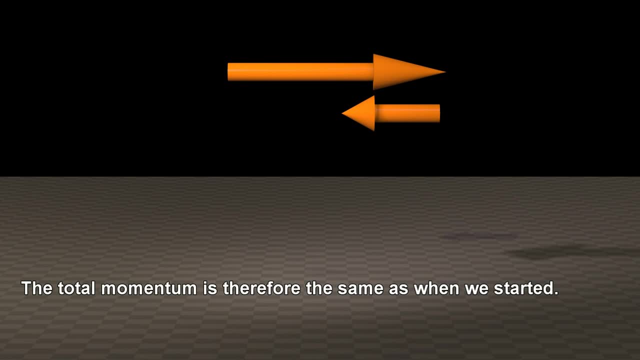 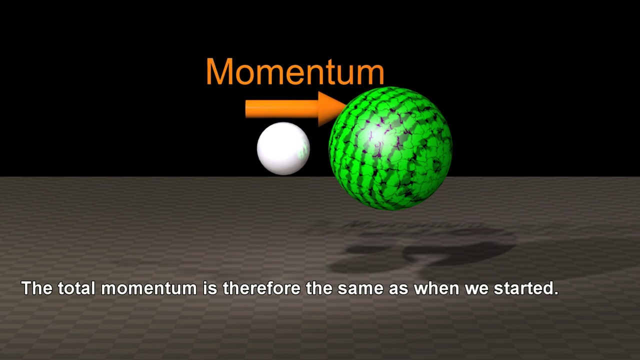 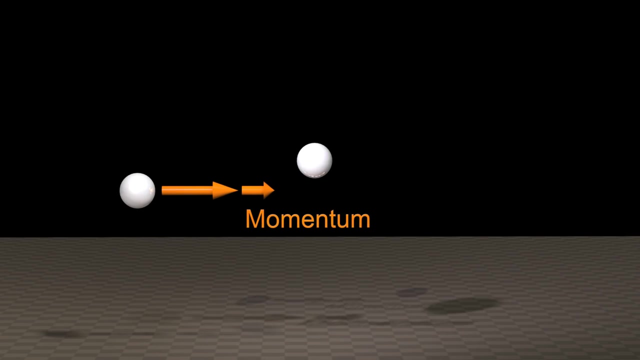 The total momentum is therefore the same as when we started. In this case, the green object is moving slowly, but its momentum is large due to the fact that it has a large mass. Objects can have momentum in more than one direction. In this case, the green object is moving slowly, but its momentum is large due to the fact that it has a large mass. 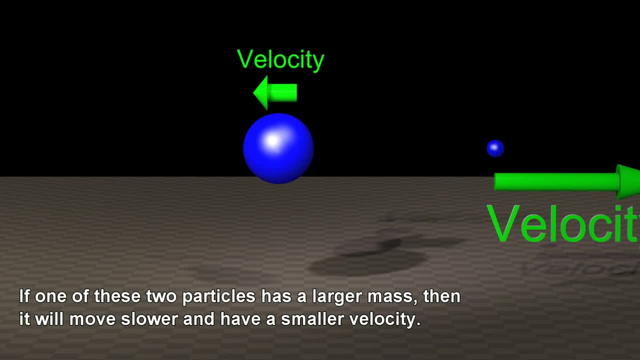 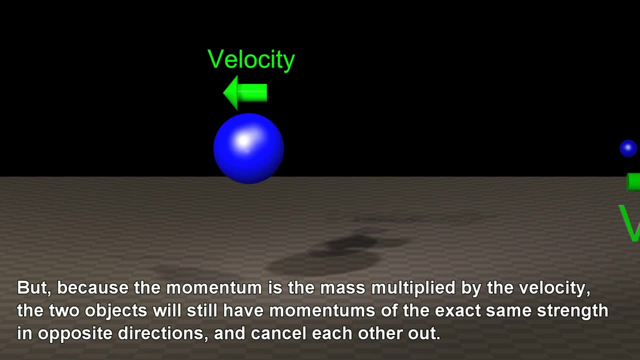 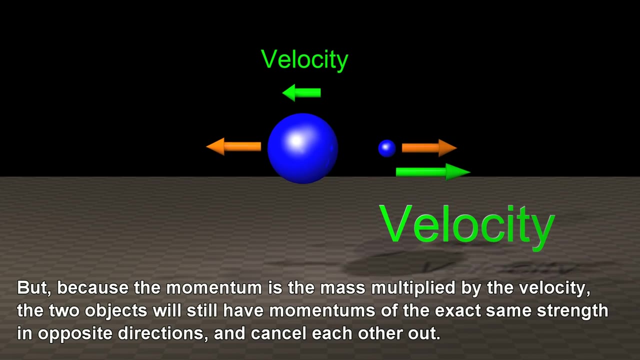 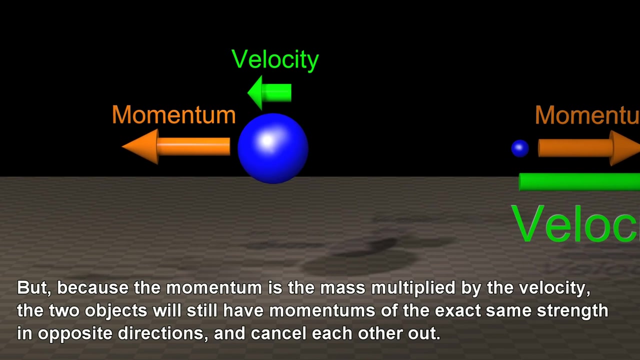 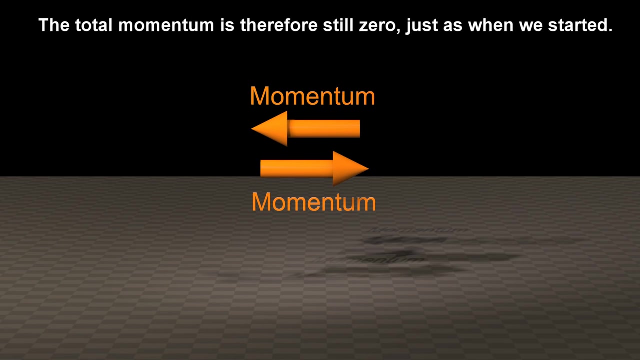 But because the momentum is the mass multiplied by the velocity, the two objects will still have momentums of the exact same strength in opposite directions and cancel each other out. The total momentum is therefore still zero, just as when we started. When one object collides with another, the momentum of one object can be transferred. 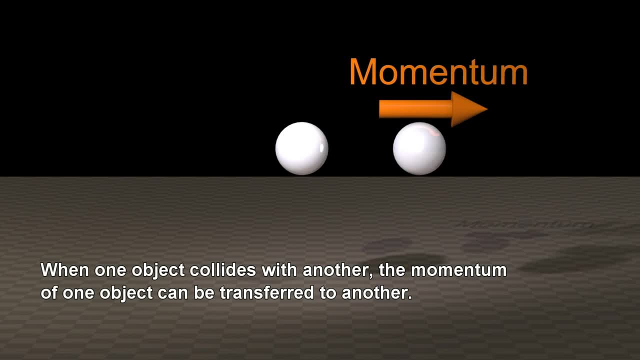 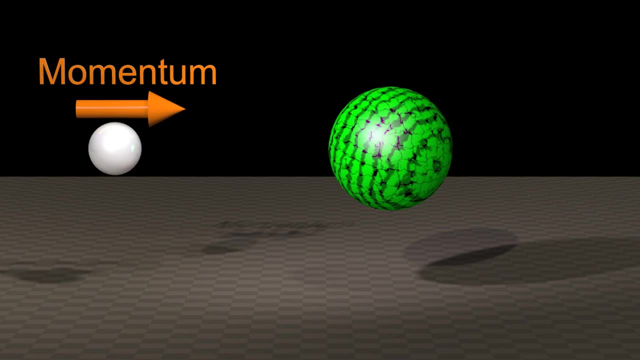 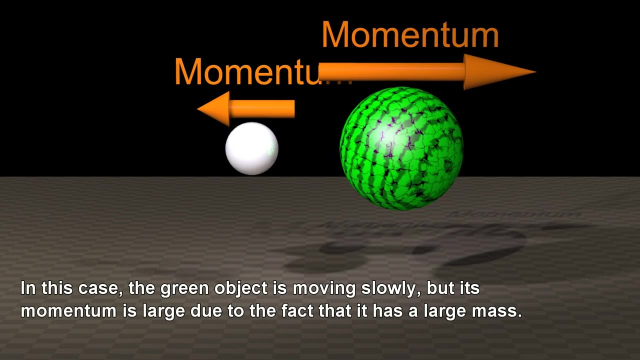 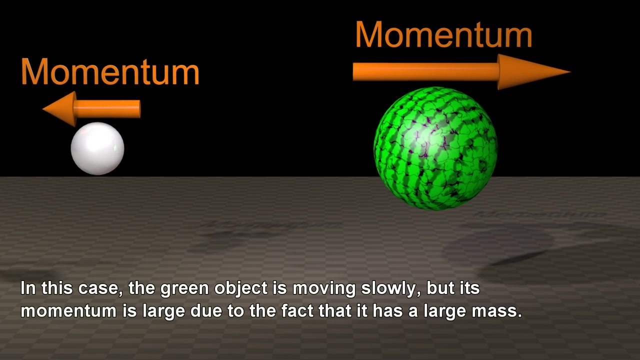 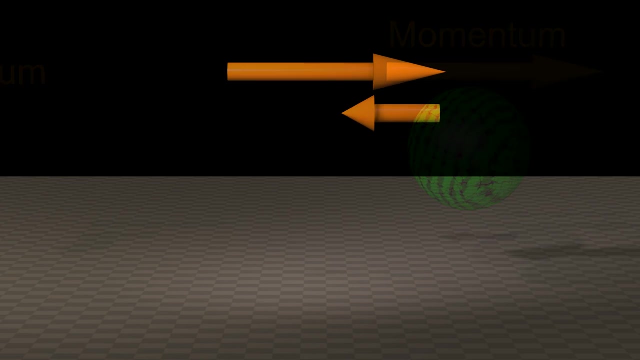 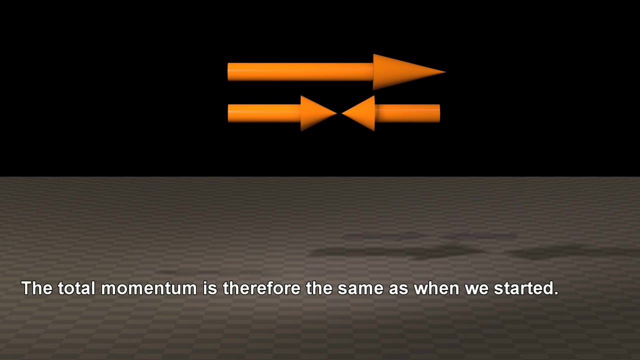 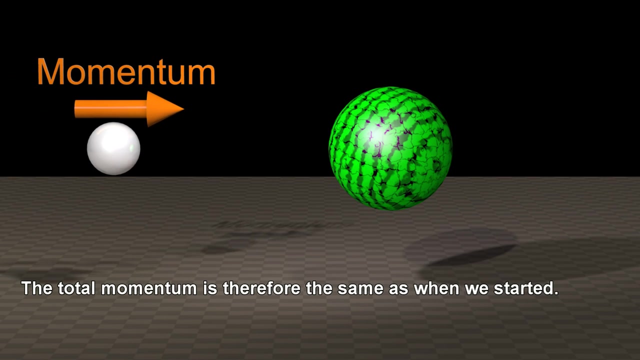 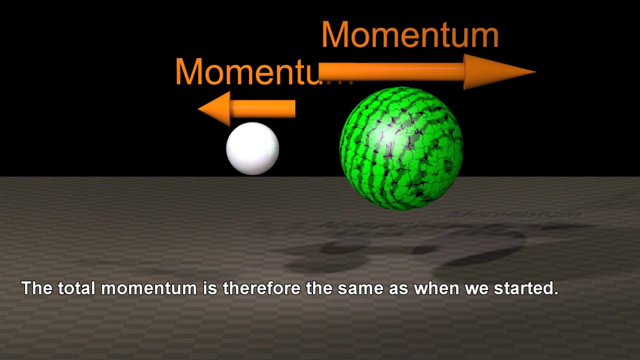 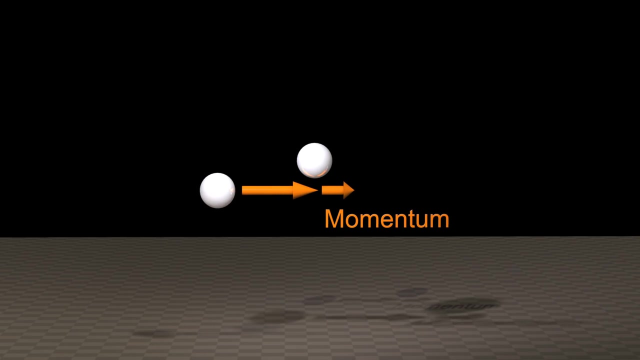 to another. In this case, the green object is moving slowly, but its momentum is large due to the fact that it has a large mass. The total momentum is therefore the same as when we started. Objects can have momentum in more than one direction. 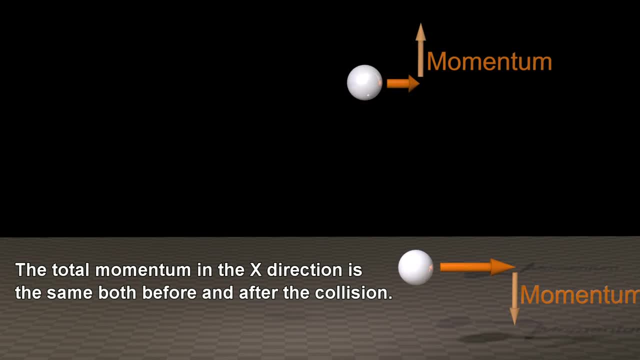 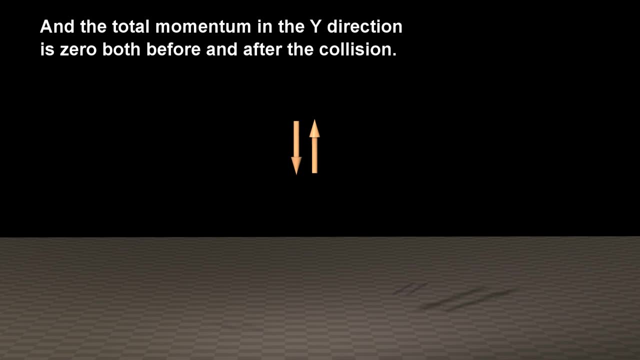 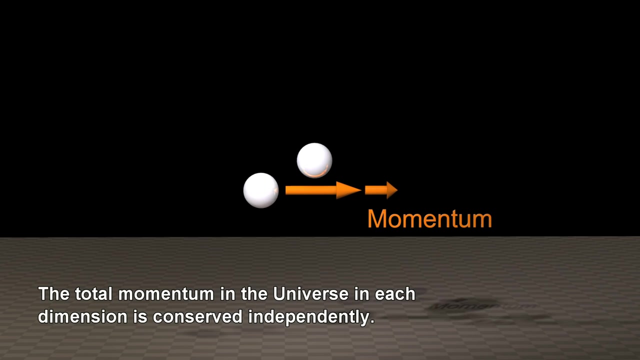 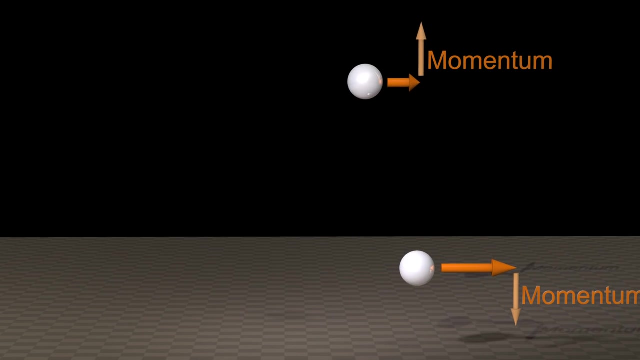 The total momentum in the X direction is the same both before and after the collision And the total momentum in the Y direction is zero both before and after the collision. The total momentum in the universe, in each dimension, is conserved independently. Now suppose that we have an object. 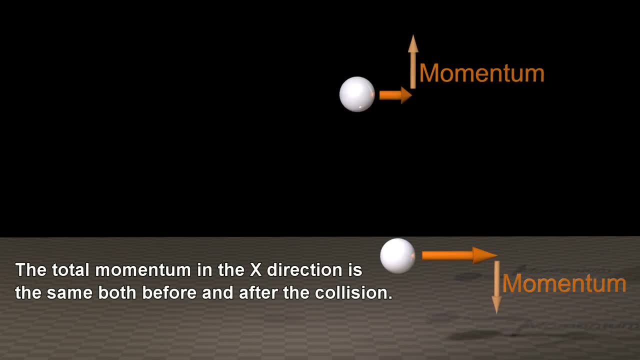 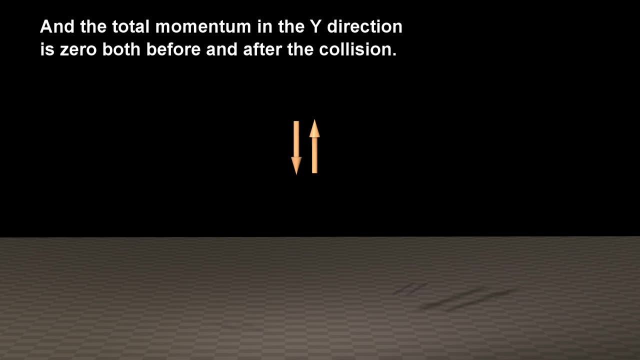 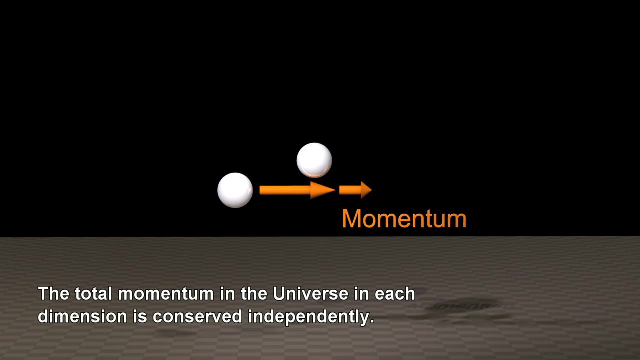 The total momentum in the X direction is the same both before and after the collision And the total momentum in the Y direction is zero both before and after the collision. The total momentum in the universe in each dimension is zero, And the total momentum in the universe in each dimension is zero both before and after the collision. 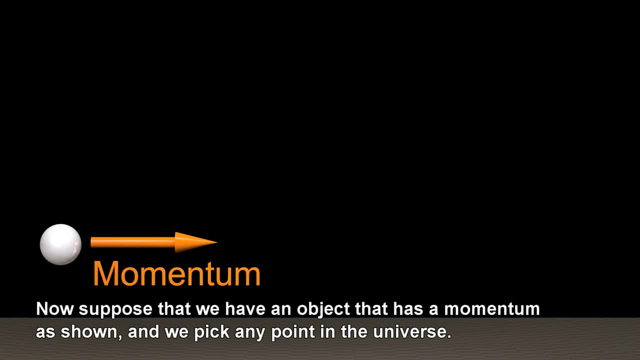 Now suppose that we have an object that has a momentum, as shown, and we pick any point in the universe. The distance between this point and the object can be measured. It can be represented by this arrow. This arrow and the arrow for momentum form a parallelogram. 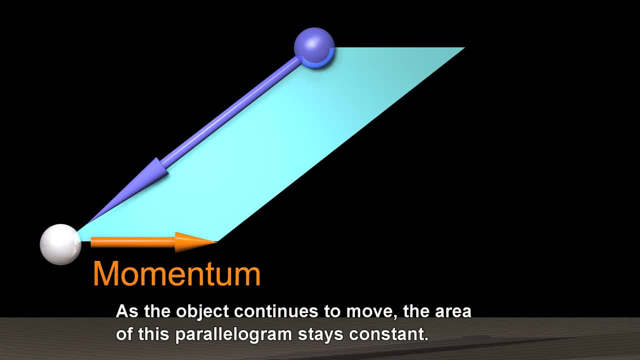 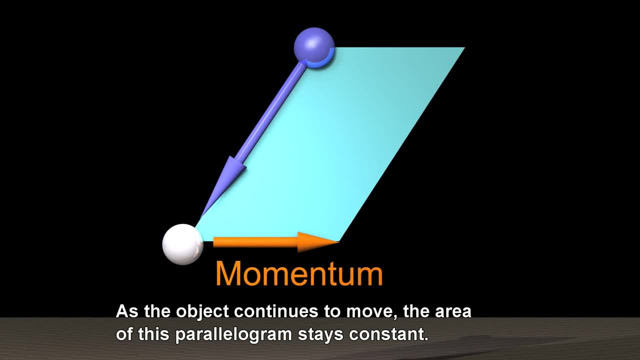 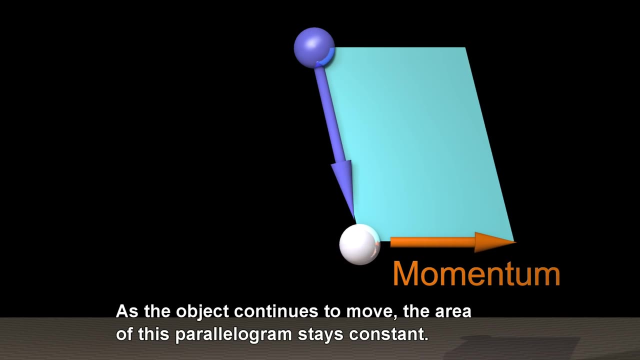 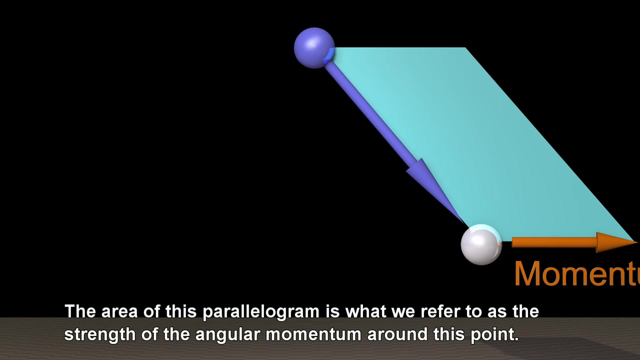 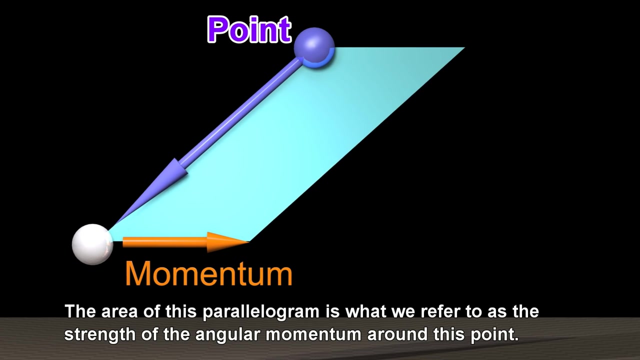 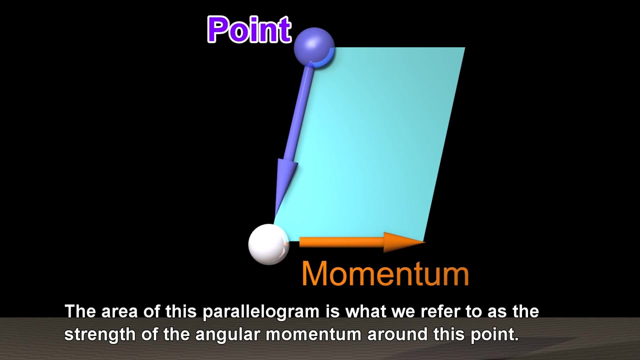 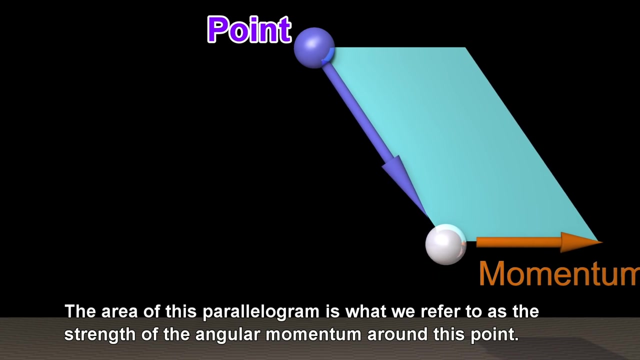 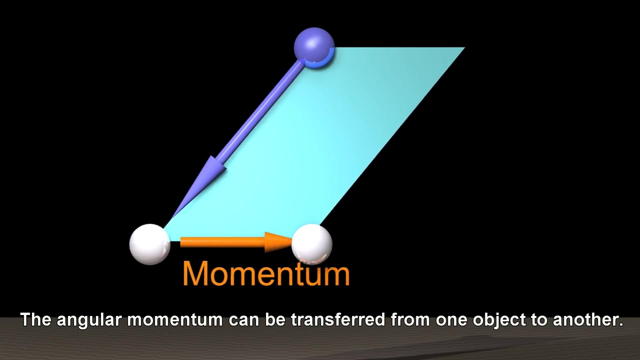 As the object continues to move, the area of this parallelogram stays constant. The area of this parallelogram is what we refer to as the strength of the angular momentum. around this point, The angular momentum can be transferred from one object to another. 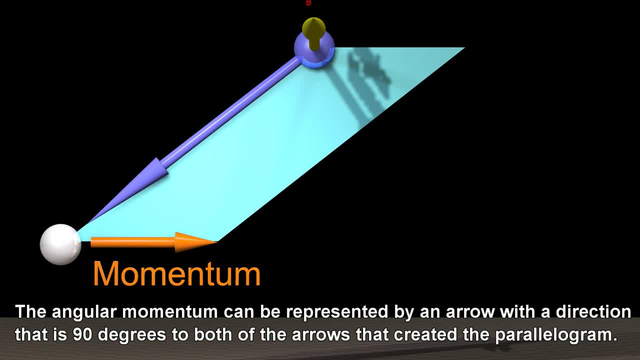 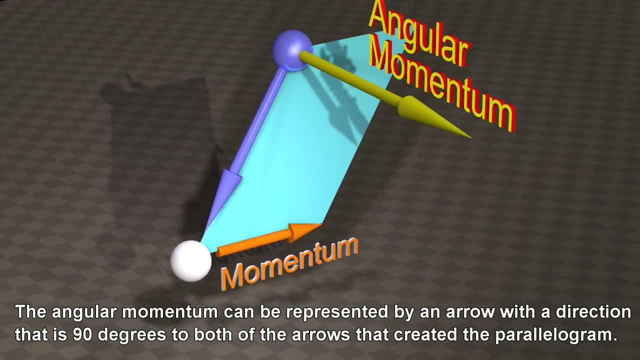 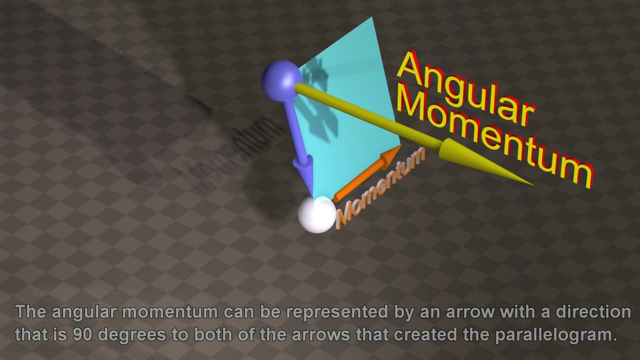 The angular momentum can be represented by an arrow, which is the strength of the angular momentum around this point, with a direction that is 90 degrees to both of the arrows that created the parallelogram. The length of the arrow represents the strength of the angular momentum. 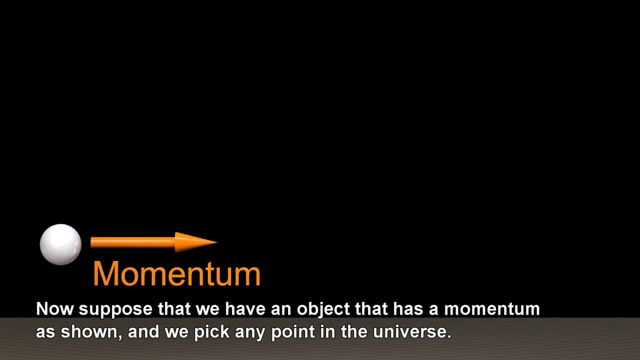 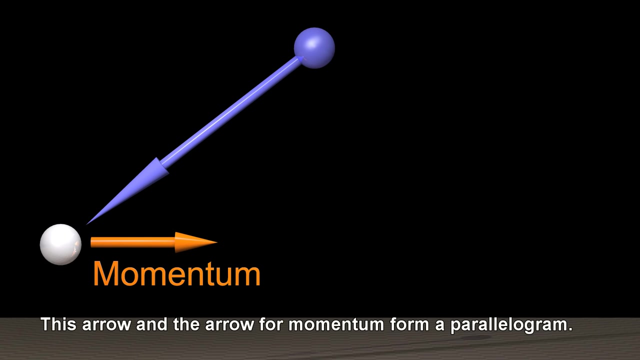 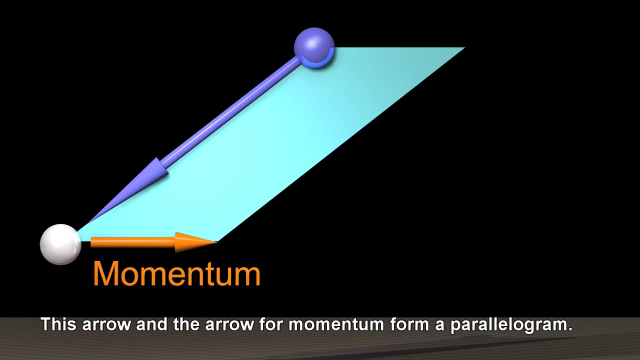 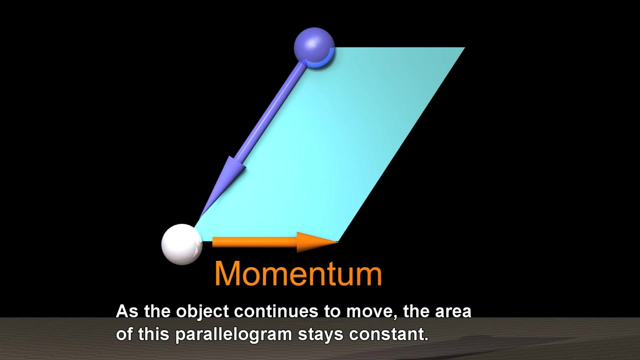 Object That has a momentum, as shown, and we pick any point in the universe, The distance between this point and the object can be represented by this arrow. This arrow and the arrow for momentum form a parallelogram. As the object continues to move, the area of this parallelogram stays constant. 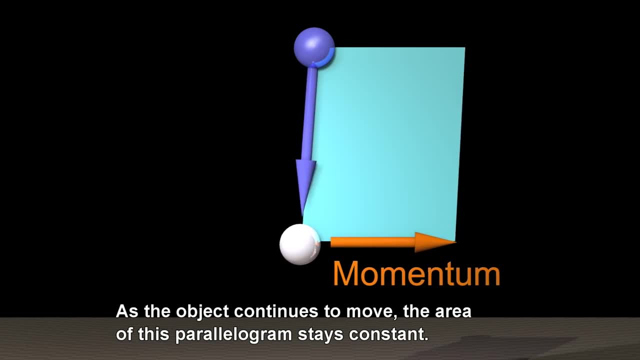 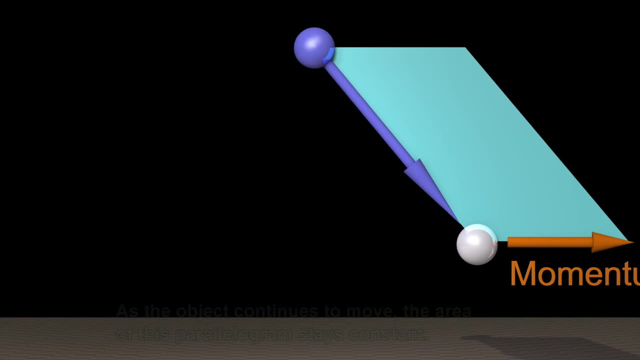 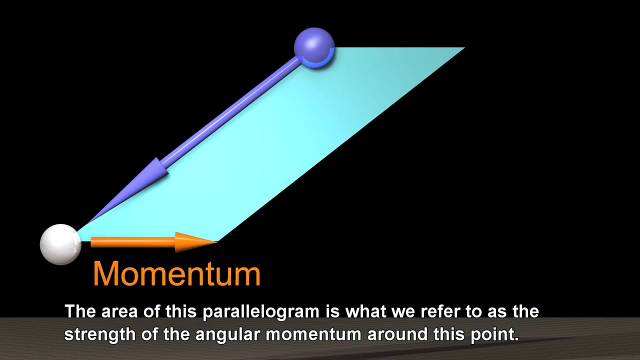 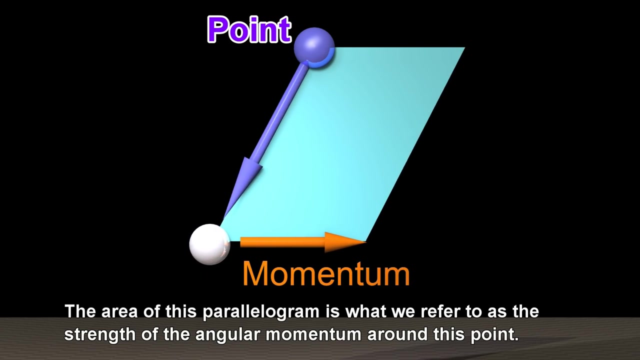 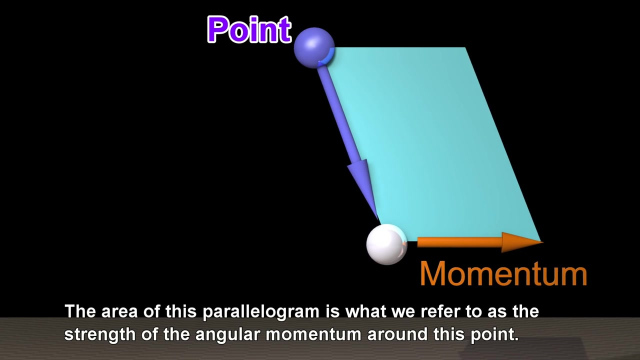 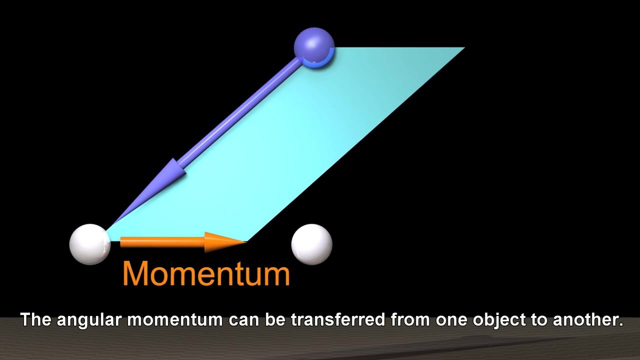 Object, And this arrow and the arrow and this point also apply to one another. Parallelogram ook Carol Knock Сов. The diagram is what we refer to as the strength of the angular momentum. around this point, The angular momentum can be transferred from one object to another. 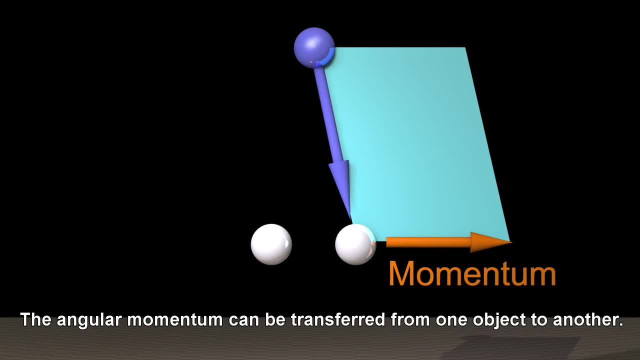 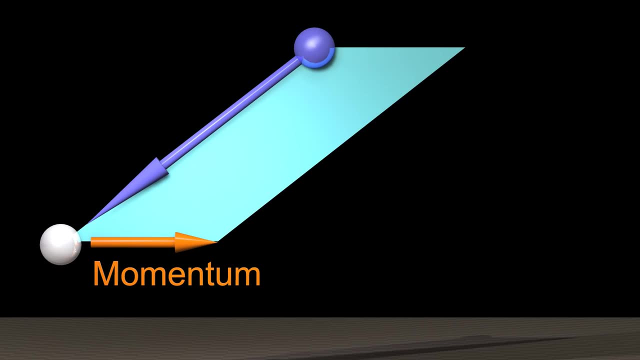 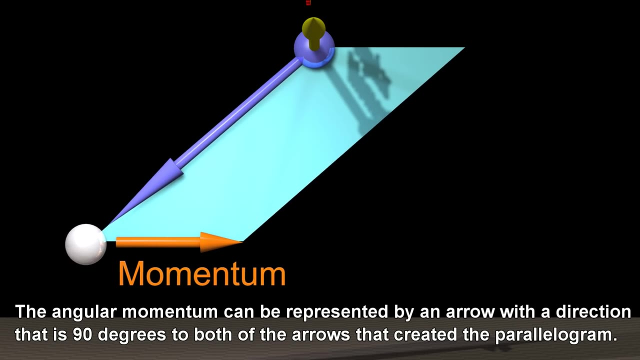 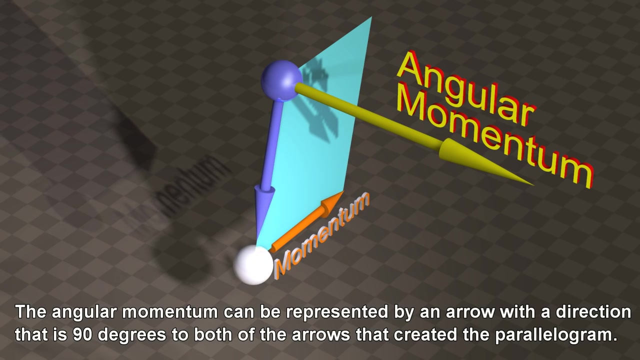 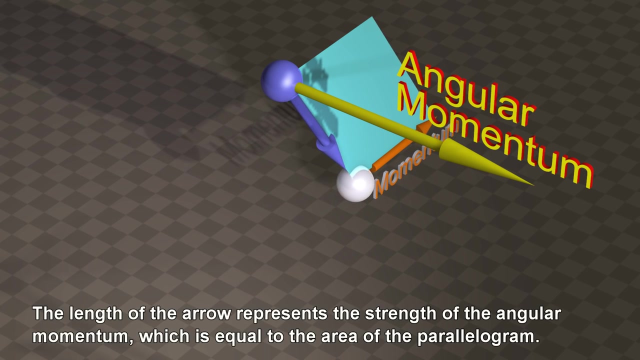 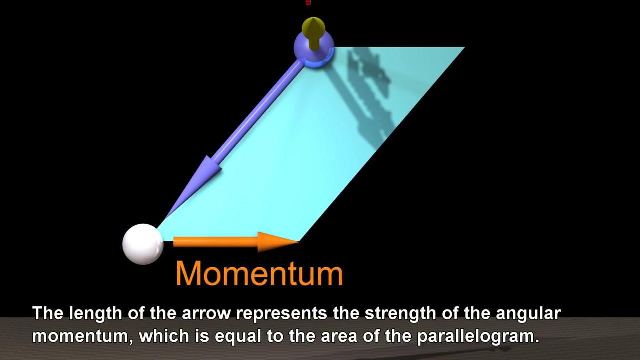 The angular momentum can be represented by an arrow with a direction that is 90 degrees to both of the arrows that created the parallelogram. The length of the arrow represents the strength of the angular momentum, which is equal to the area of the parallelogram. 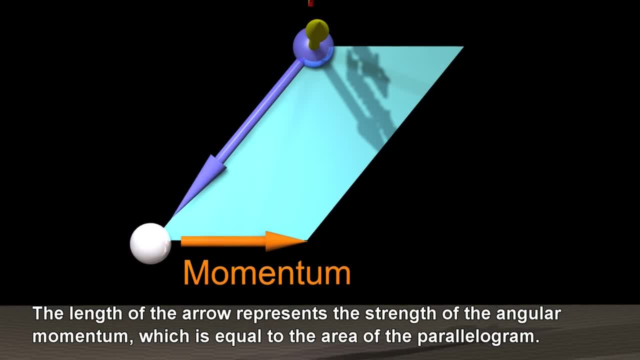 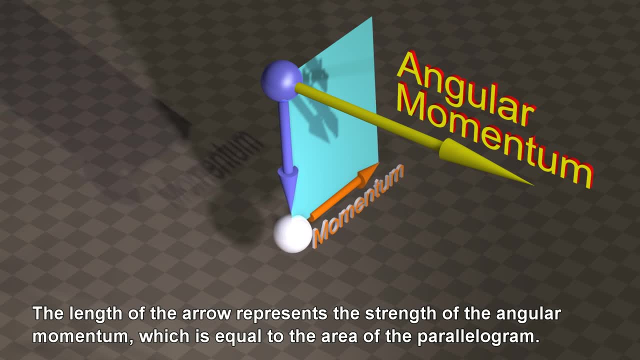 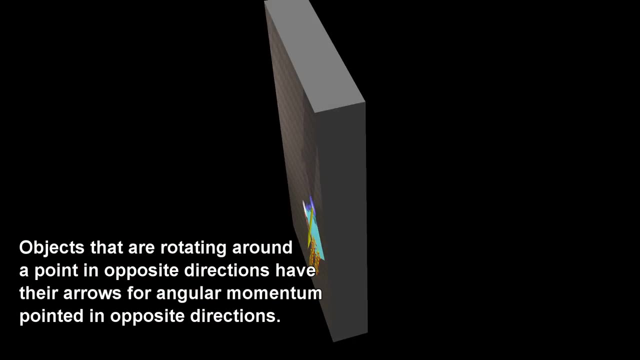 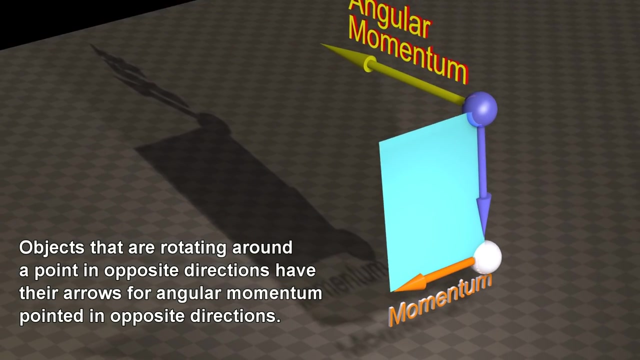 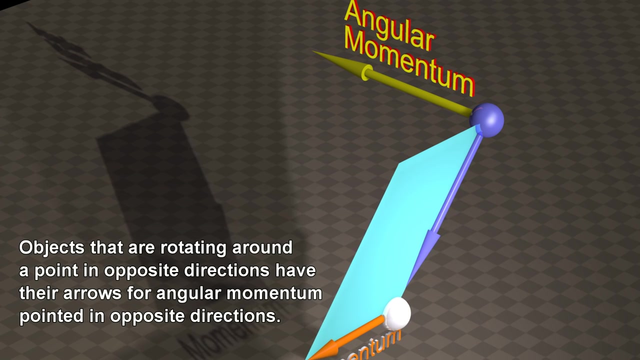 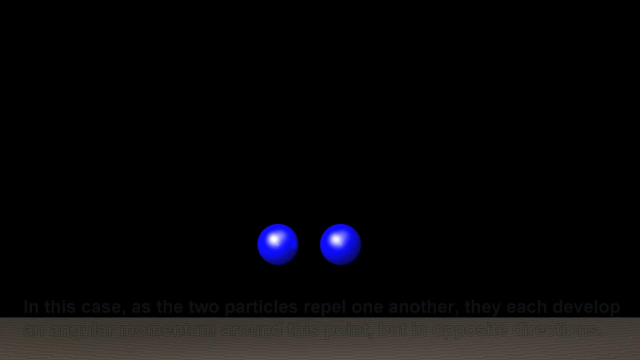 which is equal to the area of the parallelogram. Objects that are rotating around a point in opposite directions have their arrows for angular momentum pointed in opposite directions. In this case, as the two particles repel one another, they each develop an angular momentum around this point. 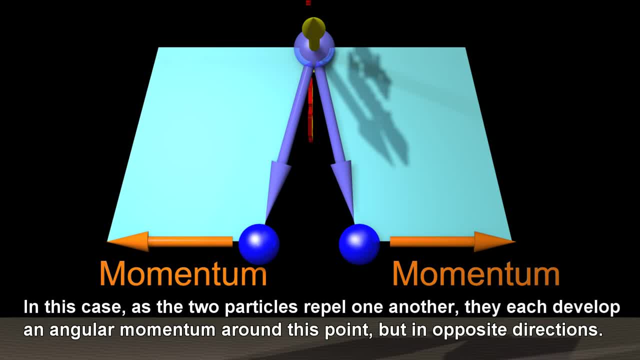 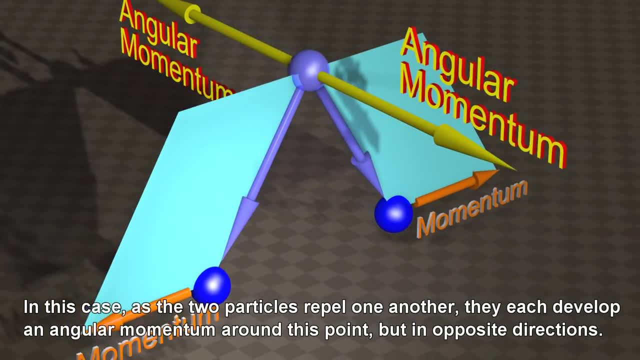 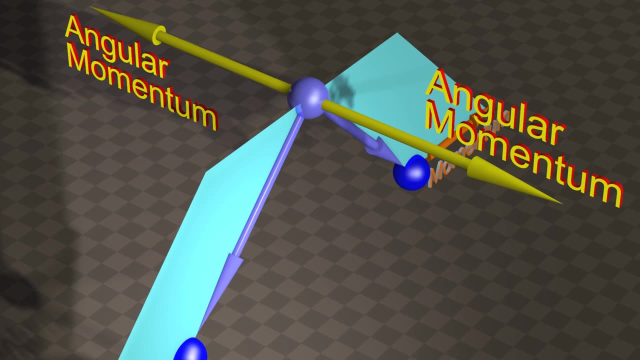 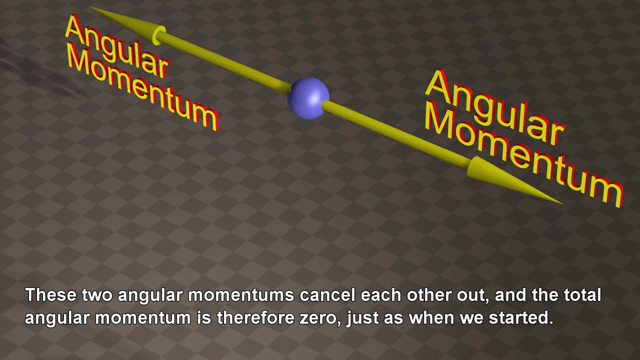 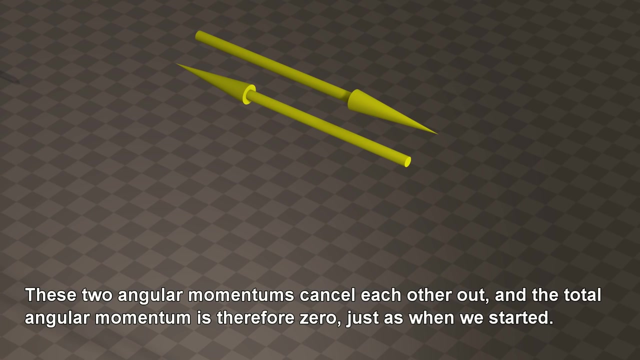 but in opposite directions. These two angular momentums cancel each other out And the total angular momentum is therefore zero, just as when we started. For any point we pick, the total angular momentum of the Universe around, that point will always stay constant. 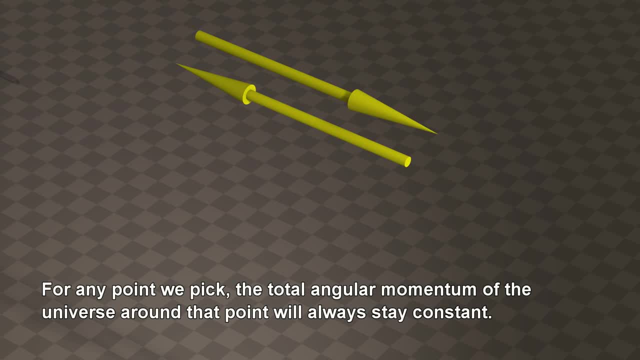 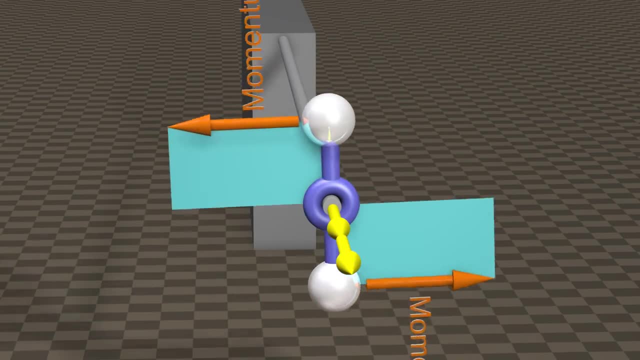 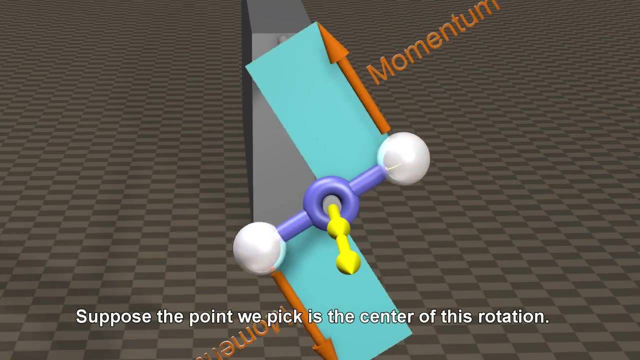 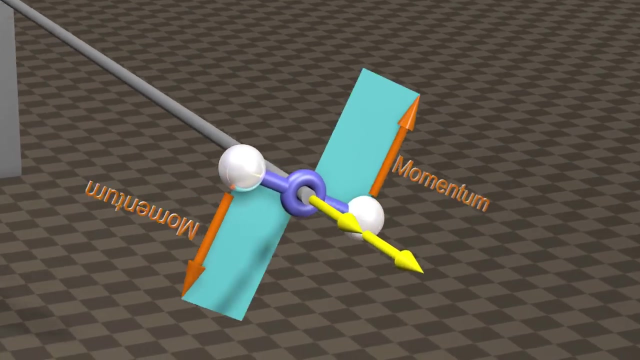 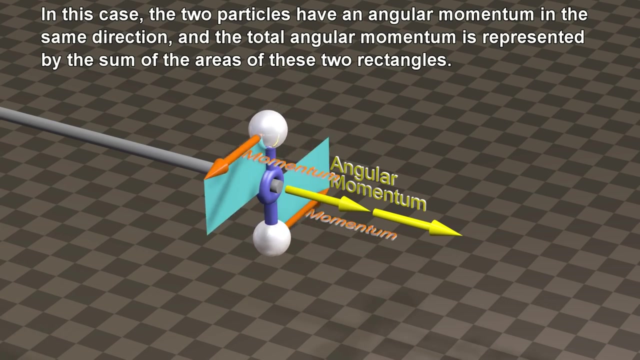 Suppose the point we pick is the center of this rotation. In this case the two particles have an angular momentum in the same direction and the total angular momentum is represented by the sum of the areas of these two rectangles. The angular momentum stays constant. 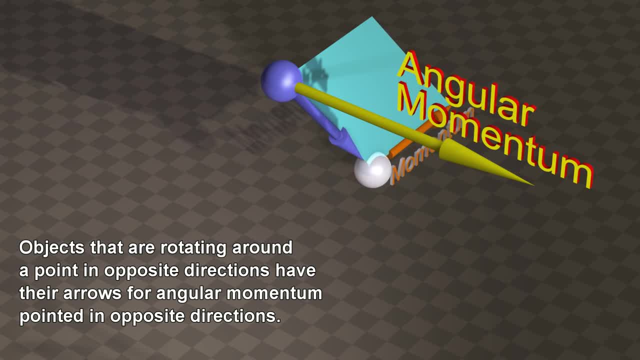 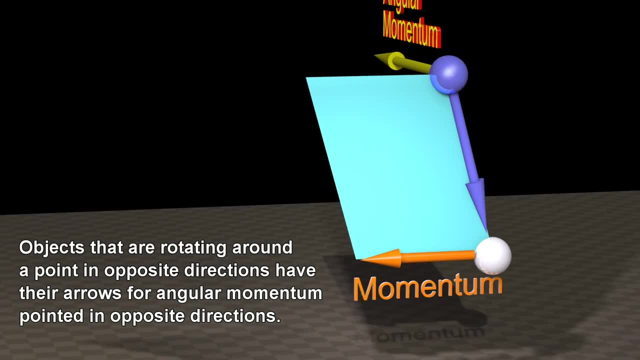 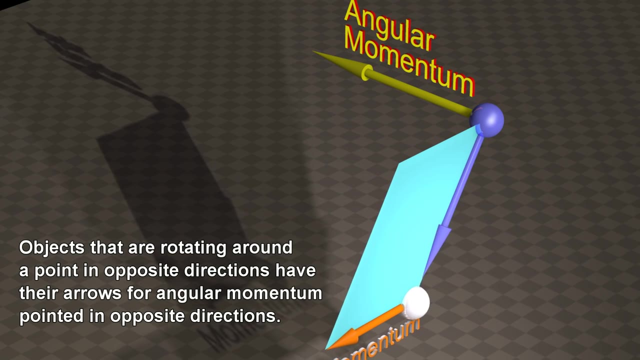 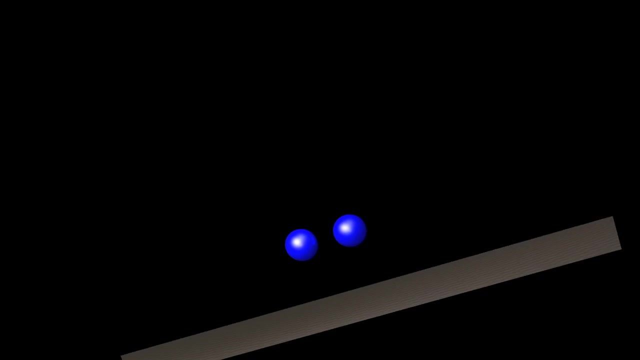 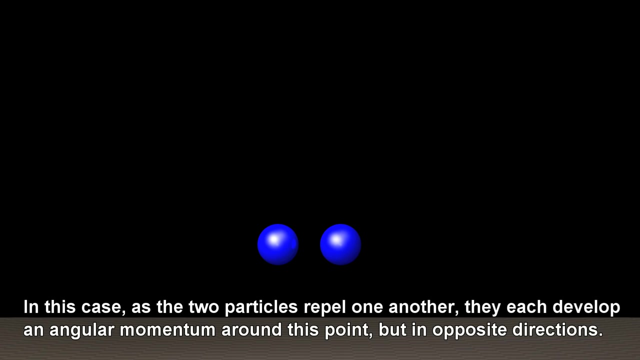 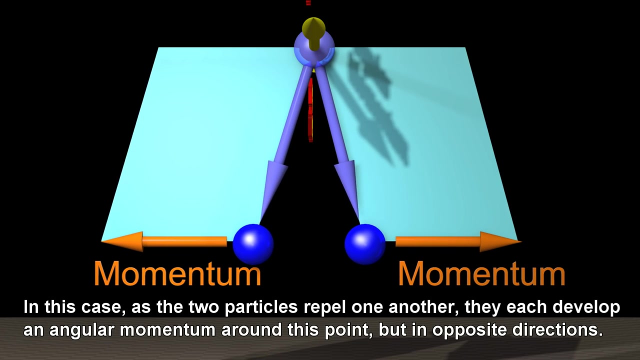 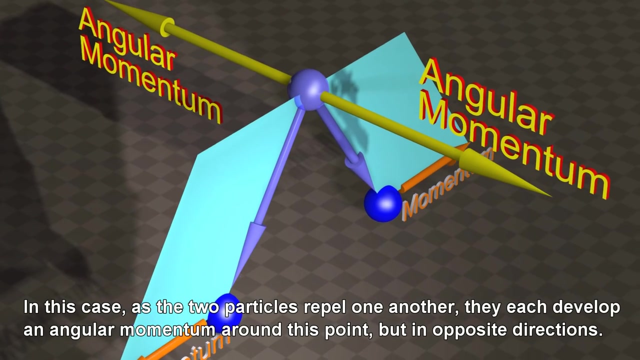 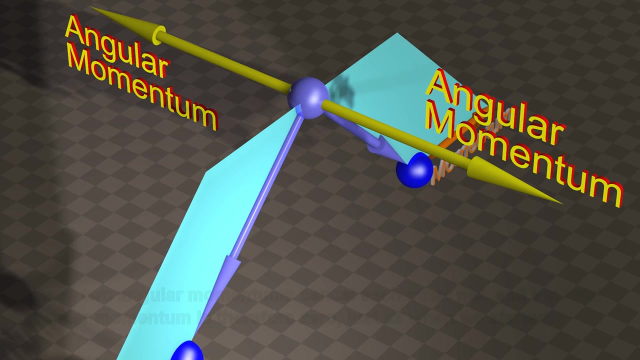 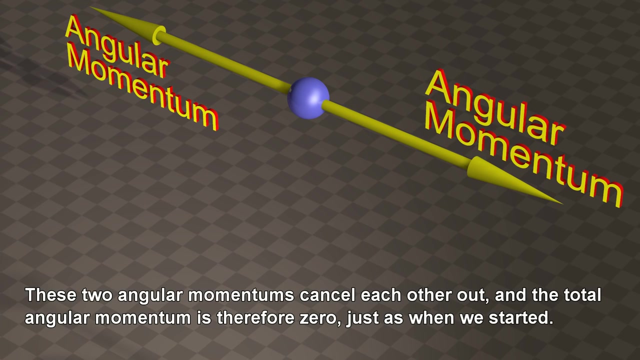 Objects that are rotating around a point in opposite directions have their arrows for angular momentum pointed in opposite directions. In this case, as the two particles repel one another, they each develop an angular momentum around this point, but in opposite directions. These two angular momentums cancel each other out, and the total angular momentum is therefore zero, just as when we started. 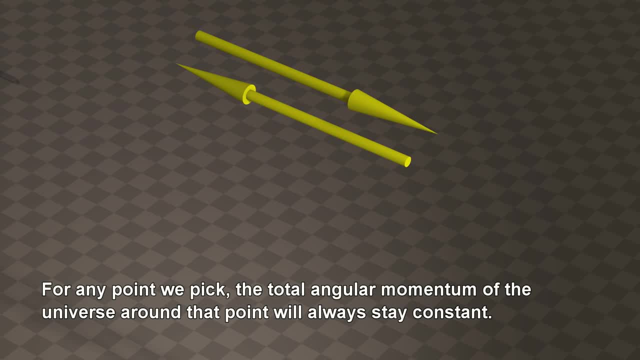 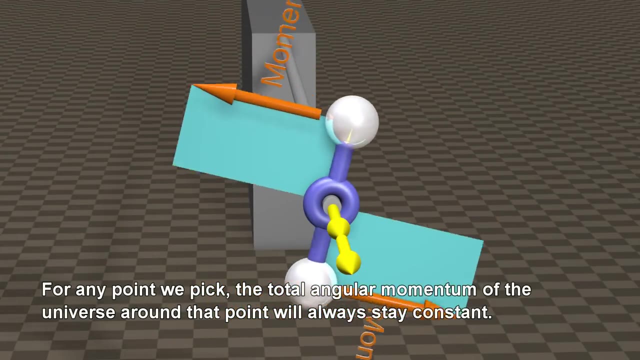 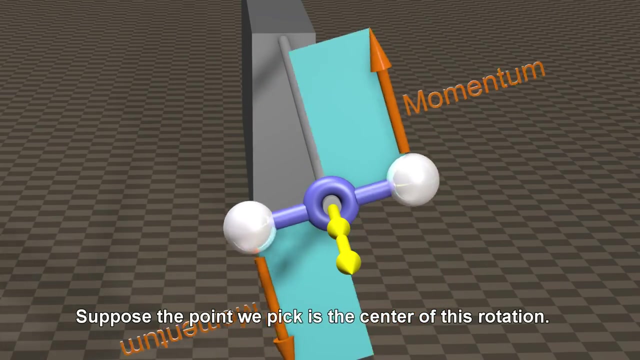 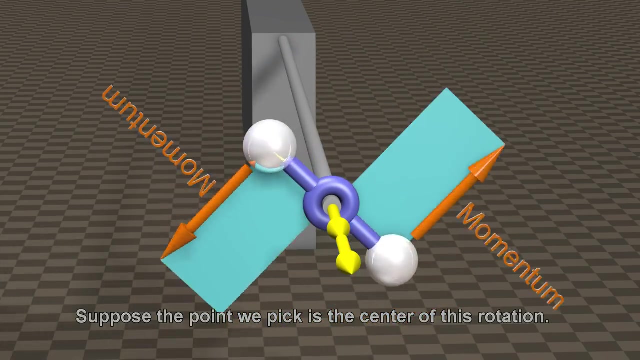 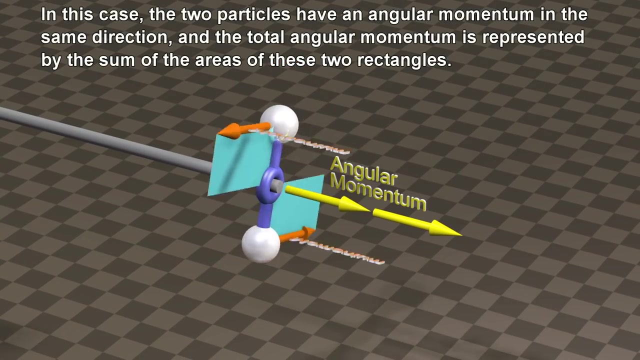 For any point we pick. For any point we pick, the total angular momentum of the universe around that point will always stay constant, Suppose the point we pick is the center of this rotation. In this case, the two particles have an angular momentum in the same direction and the total angular momentum is represented by the sum of the areas of these two rectangles. 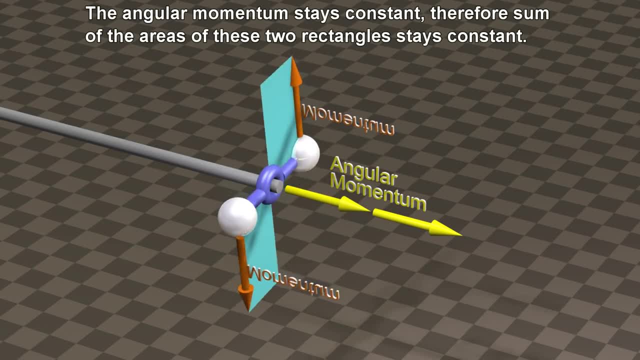 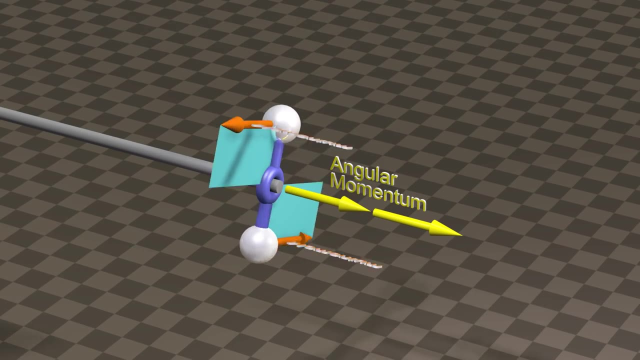 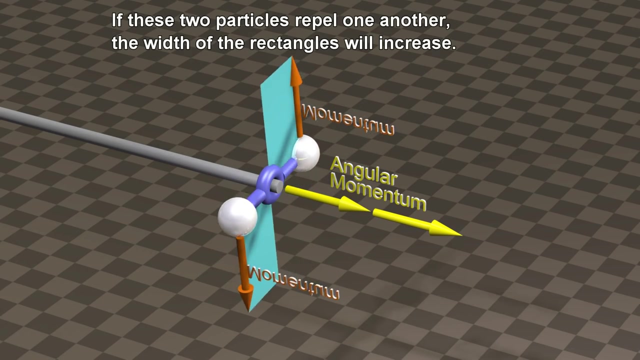 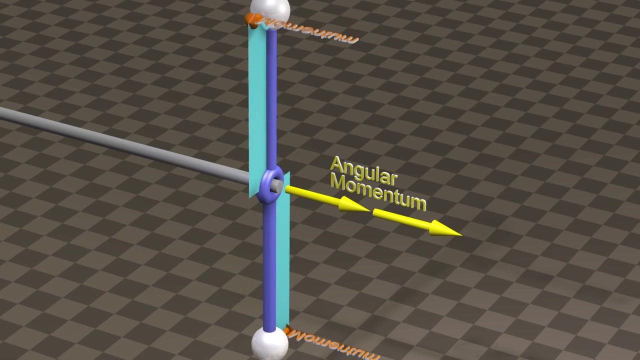 The angular momentum stays constant. Therefore, the sum of the areas of these two rectangles stays constant. If these two particles repel one another, the width of the rectangles will increase. The length of the rectangles will therefore have to decrease to keep the areas of the 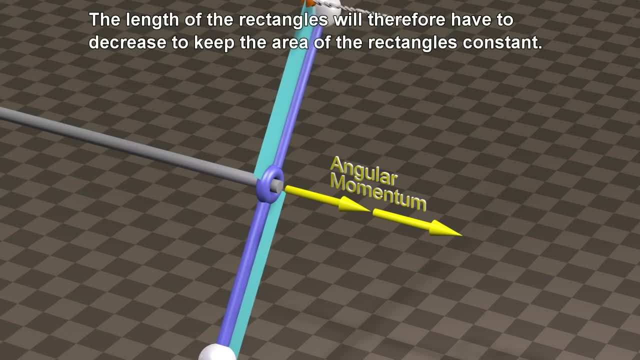 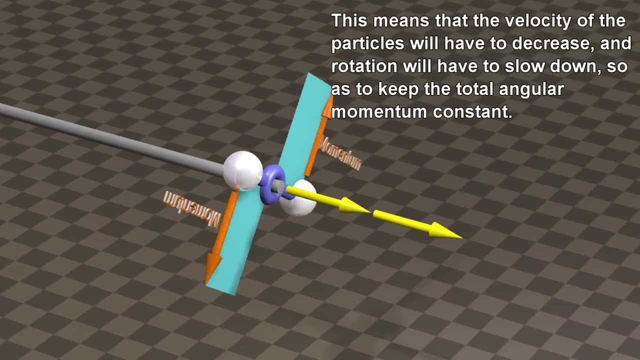 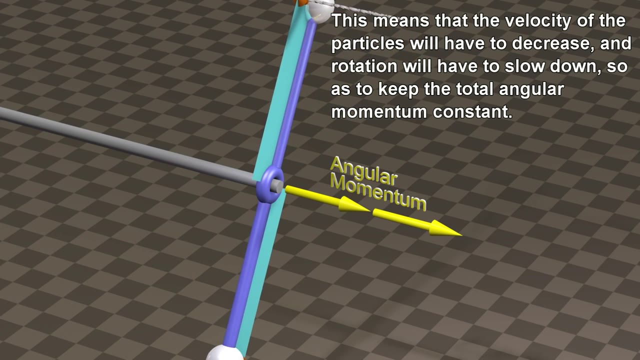 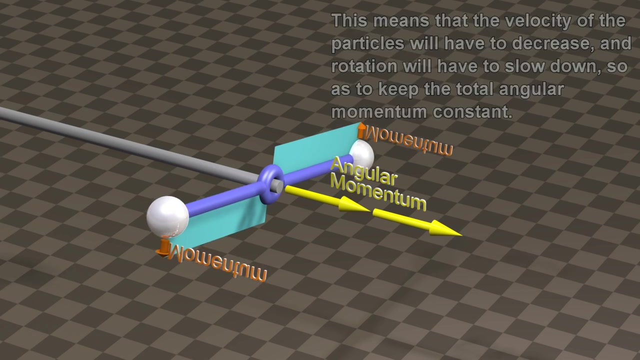 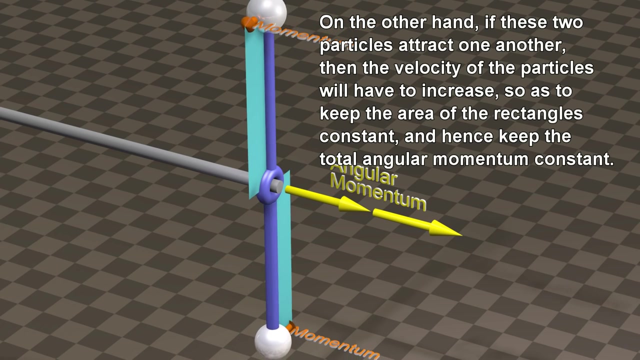 rectangles constant. This means that the velocity of the particles will have to decrease and rotation will have to slow down so as to keep the total angular momentum constant. On the other hand, if these two particles attract one another, then the velocity of